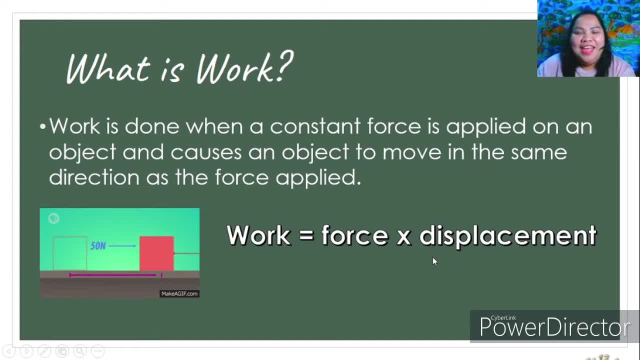 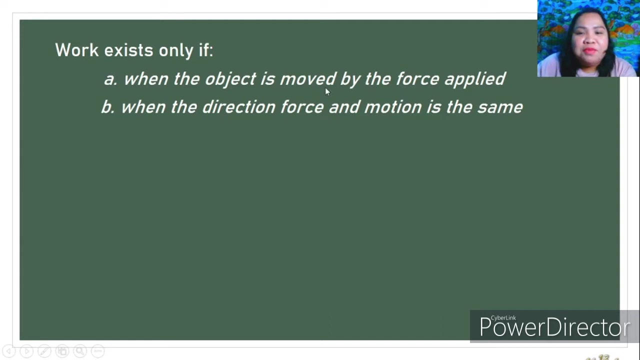 by an object's displacement. Okay, so the unit for measurement for work is Joules- We must use that- And for force, we all know that that should be in newtons. And for displacement we have meters. Okay, so work exists only if, when the object is moved by the force applied. 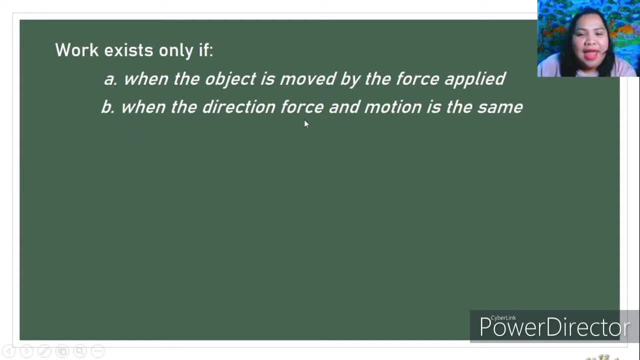 and when the direction of force and of motion is applied. This is the same. Okay, so according to physics, work would only exist if these two situations is done. Okay, I have here two examples. Let us see which man does work. 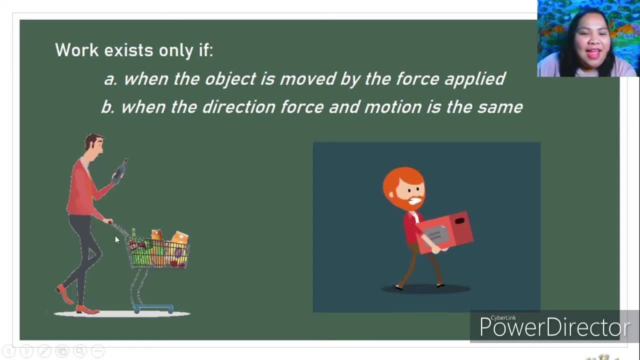 Okay, so on the left side we have a man pushing a push cart And here a man lifting a box. Okay so, let's see if there is work done. Okay, so on the left side we have a man lifting a box. 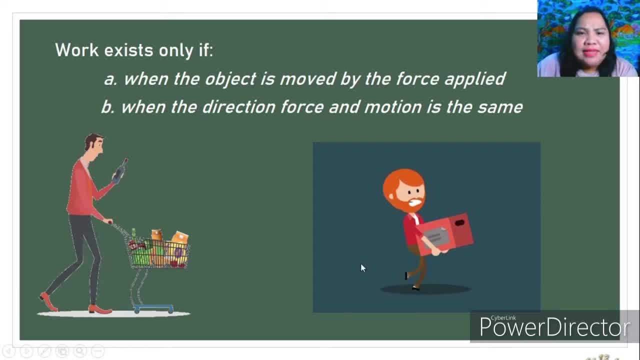 Okay, so let's see if there is work done And as the man is pushing the push cart, where is the direction of the force applied? Okay, so he is applying force towards the right. Okay, correct. And what is the direction of the motion? 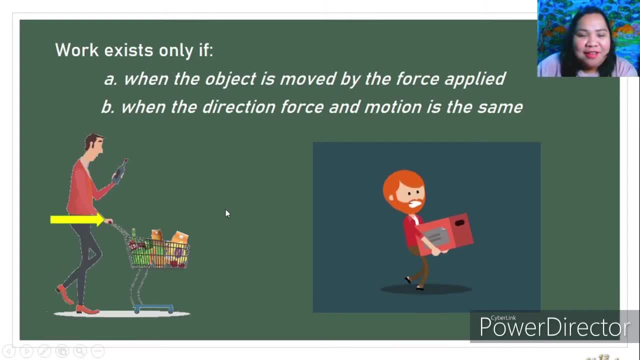 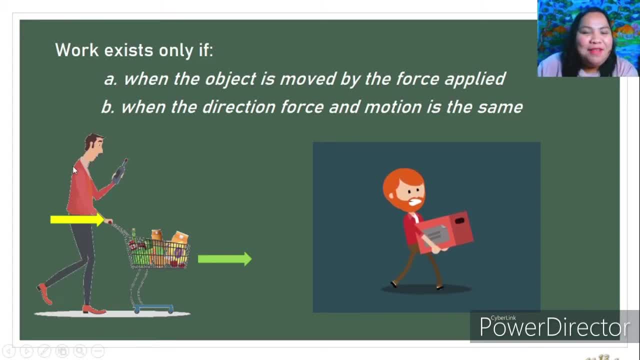 Okay, Okay, Okay, Okay, Okay, Okay, Okay. Therefore, there is work in this following example. Okay, so now we move to our next example: A man mustering all his energy to lift that box. Okay, so what is the direction of the force applied by the man? 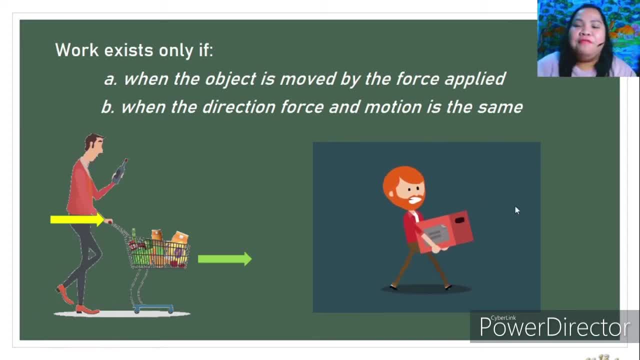 Okay, when we lift something, therefore, the force is correct, upwards, Okay, but the direction of the force is not the force applied by the man of motion is- you can see the man- that he is going towards the right. therefore, the force and the 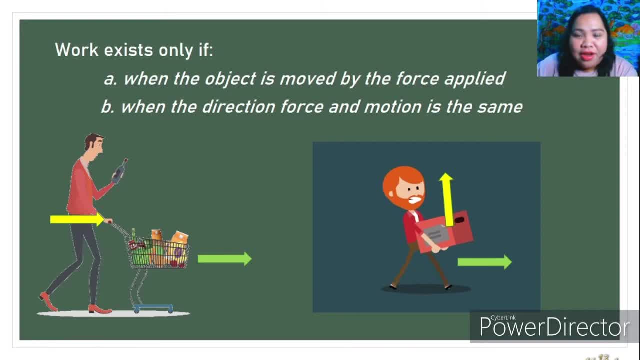 direction of motion is not on the same direction. hence we can say that in this situation, there is no work done. okay, so i hope you have, uh, you have- understand that here, um the force and the direction of the motion is in the same direction. therefore, there is work here, um the force is perpendicular. 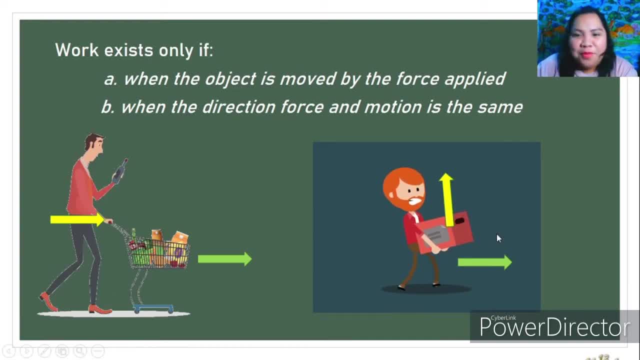 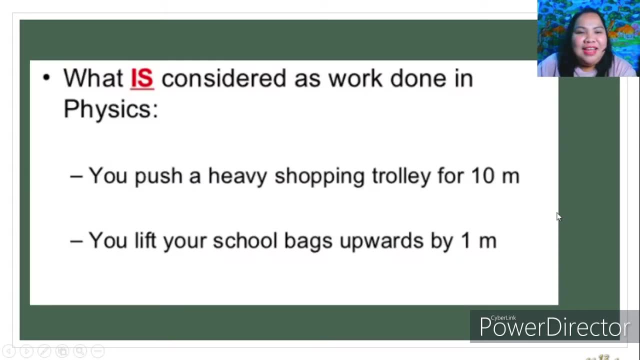 to direction of motion. therefore, there is no work done. okay, so i hope you have understand by now what is considered as work in physics. so i have here the following examples: there is work when you push a heavy shopping trolley for 10 meters. there is work. and when you lift your school bag upwards. when you lift your bag. 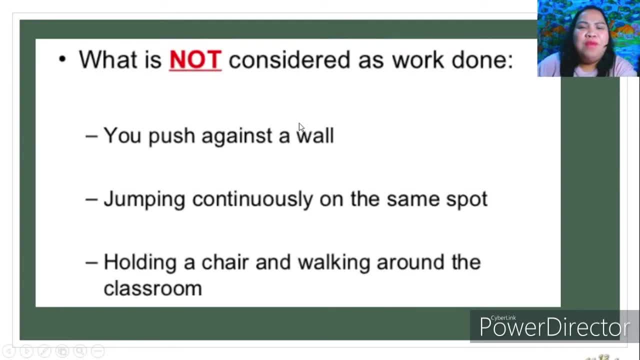 there is work done, okay. so what are the situations? when we say that work, uh, there is no work done, okay, when you push against a wall. so you muster all your energy to push that wall, but the wall is not moving, hence there is no work. remember, we need to push against a wall, and when you push against a wall, there is no work done. 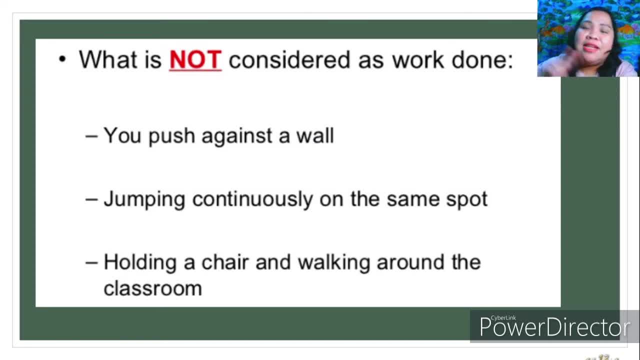 we need two values: we we need force and displacement, so the object must be moving. but here, for this example, the wall is not moving, so therefore there is no work. and another example: when we are jumping continuously on the same spot. i know it's tiring, i know, but there, according to, 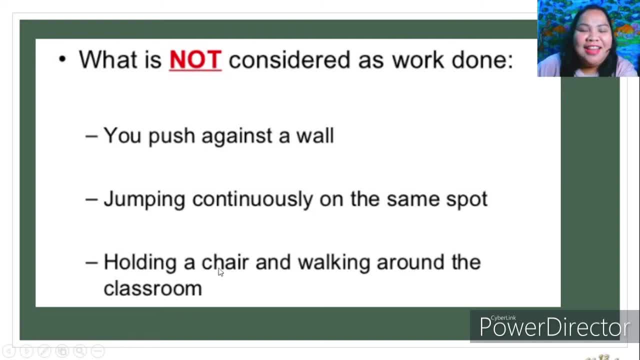 physics, there is no work done, okay. and the last one: while, uh, you, you are holding a chair while you are sitting around the classroom, so some of some of you do that inside the classroom, but as you do that, there is no work done. okay, it's because the force is not in the same direction as the 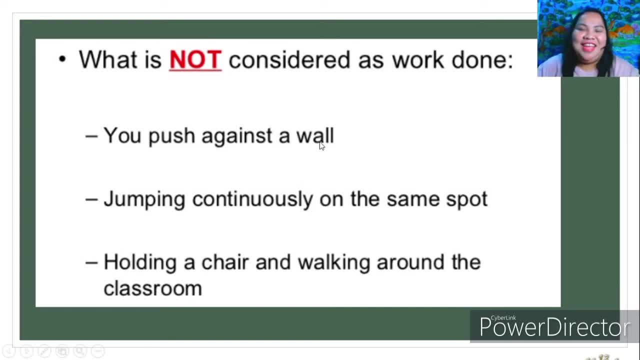 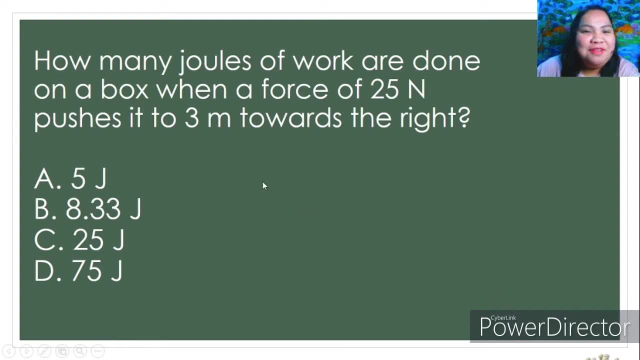 direction of motion. okay, so let's proceed to this word problem. i hope you you will solve this one. this is an easy one, okay, how many jobs do you have in your life and how many jobs do you have in your life? and how many jobs do you have in your life and how many jobs do you have in your life? 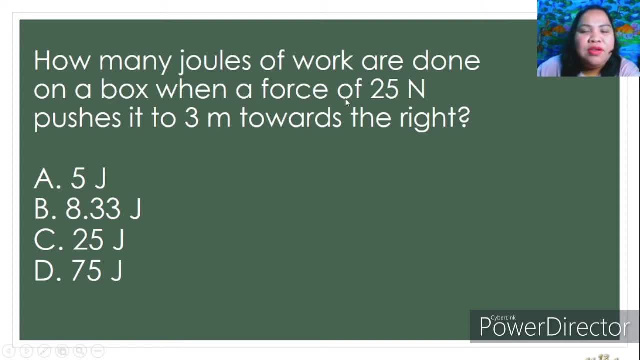 so let's look at the values. we have force here, 25 newtons, and we have the displacement three meters. okay, so, as you can remember, the formula we have: work is equals to force times a displacement. so we have to multiply the force times the displacement. so we have to multiply the force times the displacement. 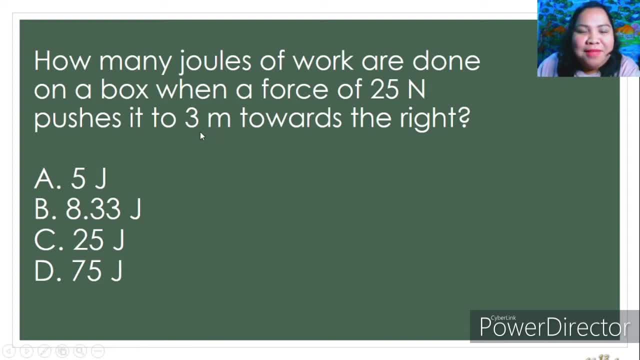 25 newtons to the displacement that is three meters we have. the correct answer is okay. the correct answer is letter d, it's 75 joules, okay. so i hope you all got that correct. you have. you only have to multiply the force and the displacement, okay. so let's proceed. so much for work, let's proceed to power. 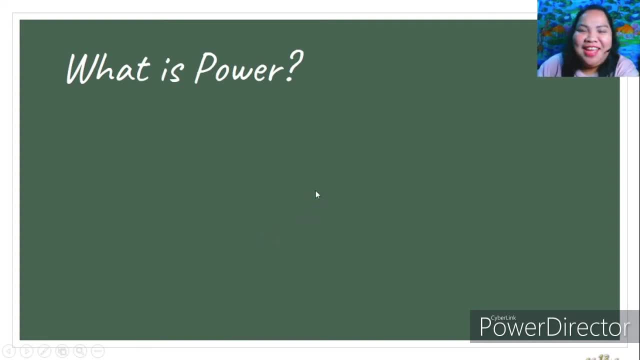 power. what is power? okay, so some of you may describe power as a magically something, something, but in physics, we will define power, or the power is defined as the rate of doing work, or the amount of work applied to an object per unit of time, and we can also say that it is. 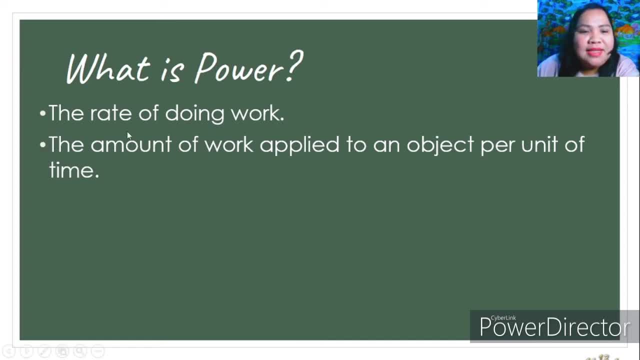 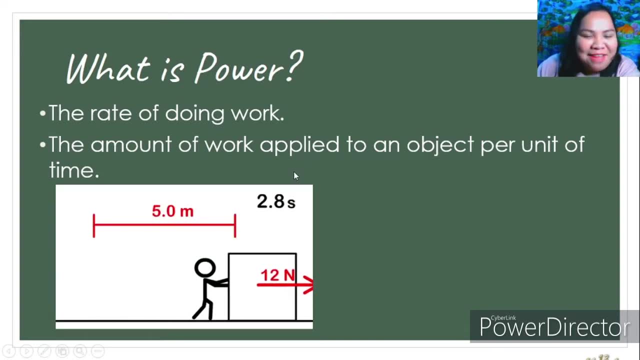 how fast we can do work and how fast we can do work, and how fast we can do work and how fast we can do work. okay, it is the rate of doing work. that is power in the world of physics. okay, so i have here a stickman. 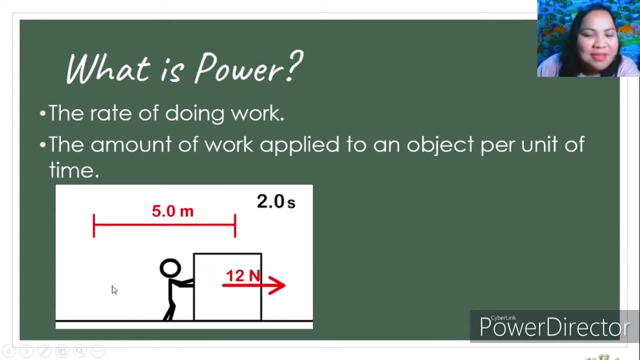 pushing a box. okay, so he applies force with 12 newtons there and moves the box to five meters in towards the right and he finishes that in three seconds. okay, so how do we solve for power? the formula for power is: power is equals to work over time, because it is the rate of doing work or how fast we do work. okay. 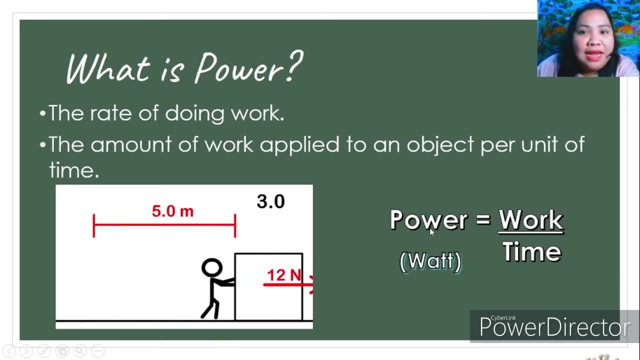 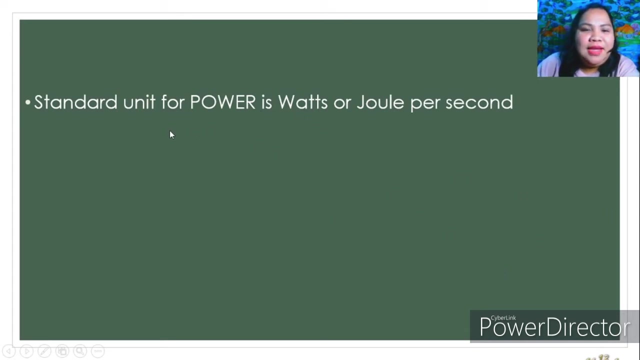 so the unit of measurement for power is watts, and for work we have joules and time. this is usually in seconds. okay, so that is the formula. in order to get power, power is equals to work over time. okay, so the standard unit for power is watts. as we stated earlier, this term is derived from james. 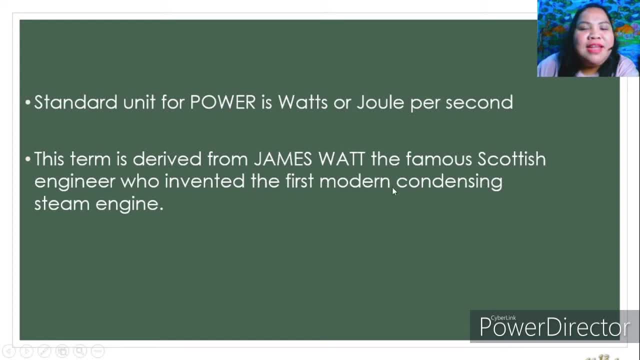 watt, the famous scottish engineer who invented the first modern condensing steam engine. and one watt is equal to one joule of work done in one second. okay, so for those of you who wanted to know, how many watts is equivalent to one whole hour of work. so the unit for power is watts and the burned and 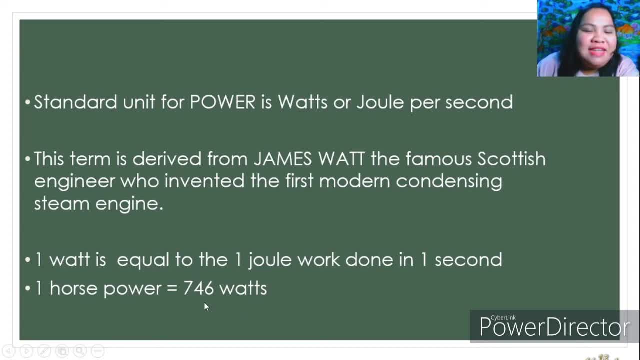 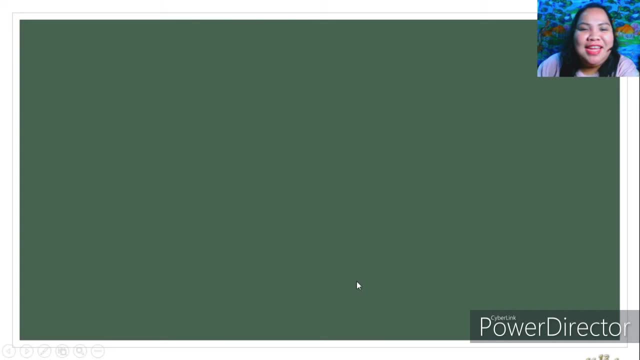 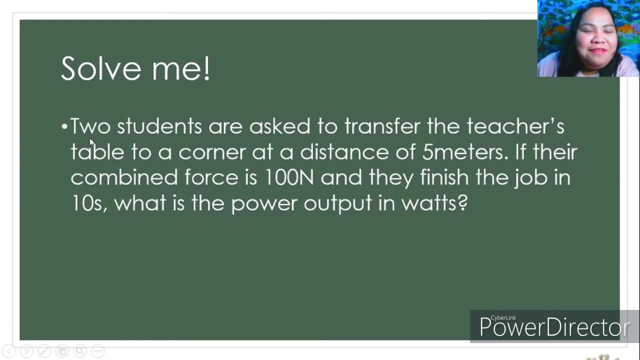 one horsepower. there we go. we have: 746 watts is equivalent to one horsepower. okay, so let's proceed. so i have here another problem for you to solve. okay, so we have two students are asked to transfer the teacher's table to a corner at a distance of five meters. if their combined force is 100. 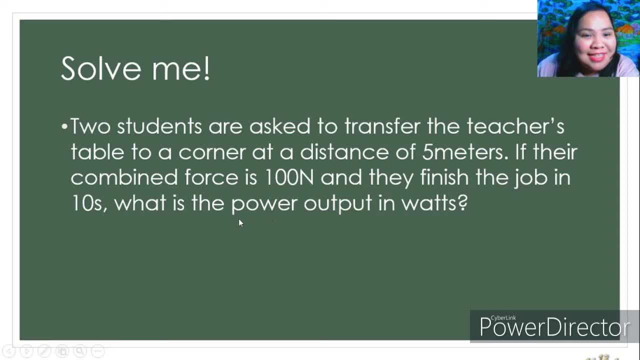 newtons and they finish the job in 10 seconds. what is the power output in watts? okay, so we all know that the formula for power is work over time. so remember, the unit of measurement for work is joules, right, but when we look at the problem, there is no value in joules, right? okay, so that. 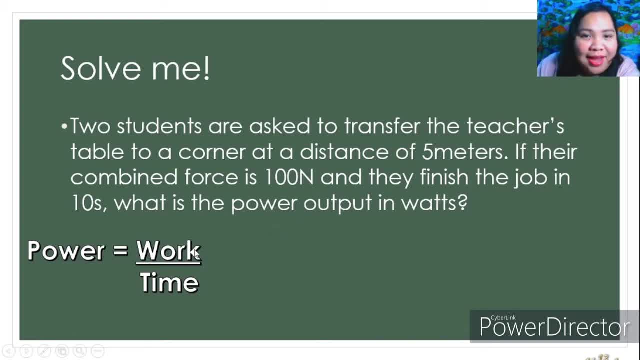 is the problem means we have to solve for work, and we know the formula for work is: work is always equal to the force and the displacement. okay, so force multiplied by the object's displacement over time. so we can also use the following formula in all in order to solve, to solve for power, okay, so let us find. 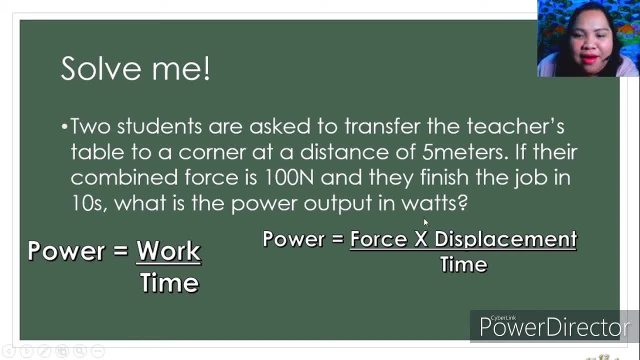 force there, that is the 100 newton there, and then multiply to the displacement that is usually in meters. we have five meters. so that means 100 newtons times five meters and we get 500 right. 100 multiplied to five, we have 500 and divided by 10 seconds, 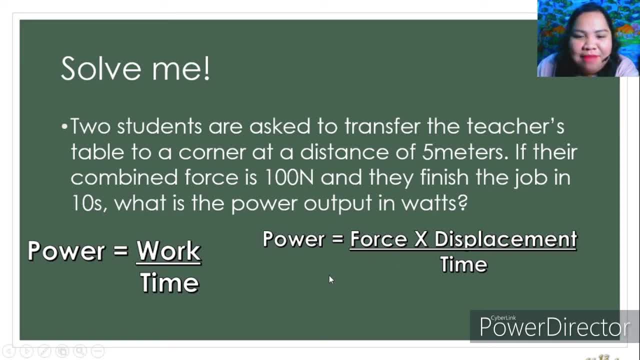 because that's the time. so 500 divided by 10, we have 50 watts, the correct answer for that problem. the power output is 50 watts, so i hope you have the same answer as we have here. okay, so now you know how to solve for work. 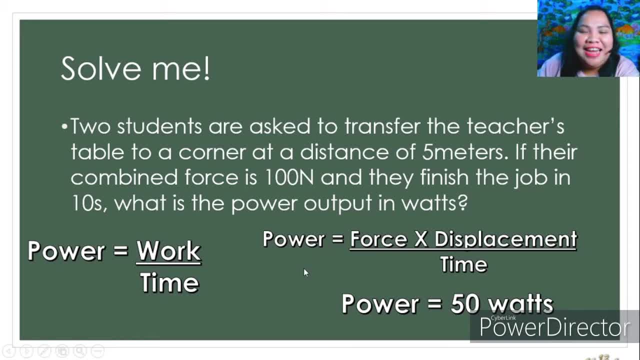 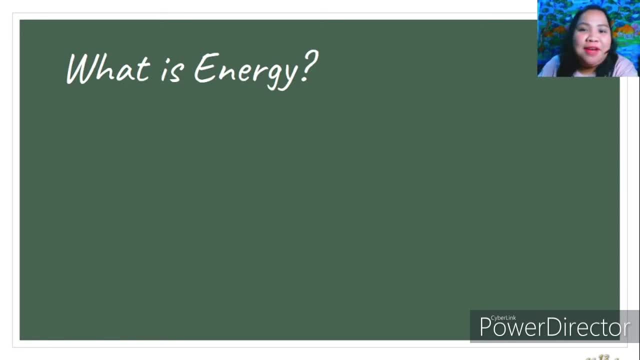 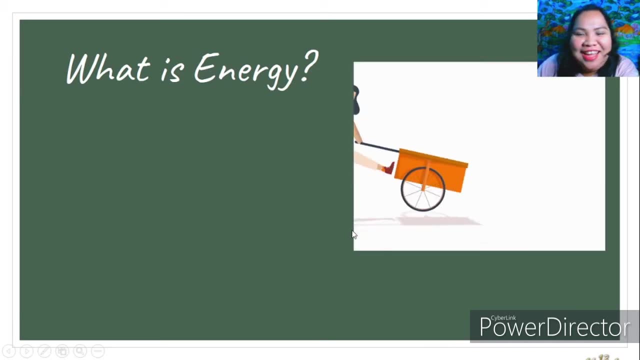 and also for power. okay, let's proceed. so after work, after power, now we will discuss about energy. so what is really energy? energy is okay. i have here an example: a lady pushing a cart with um, his, she is happily pushing a cart, okay. so in physics, energy is the. 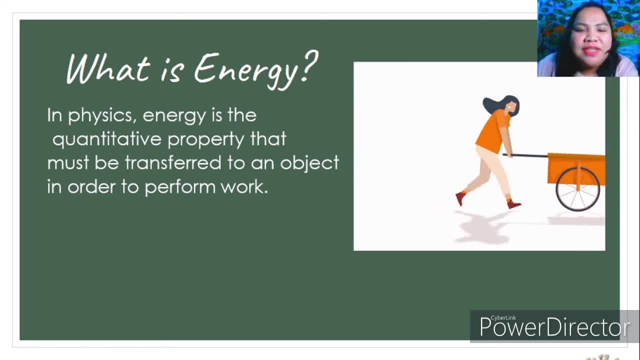 quantitative property that must be transferred to an object in order to perform work. okay, the quantitative property that must be transferred to an object in order to perform work, or, in other words, okay. in layman's term, we identify energy as the capacity or the ability to do work. okay, when you don't have energy, you. 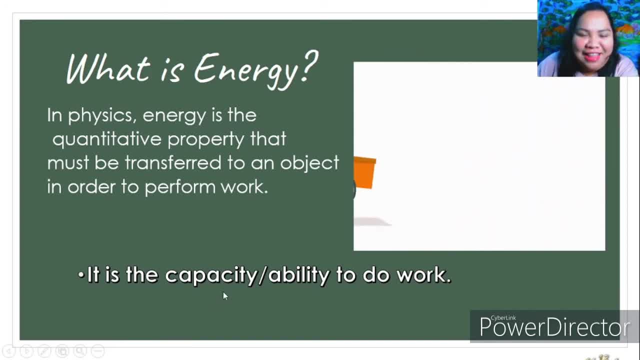 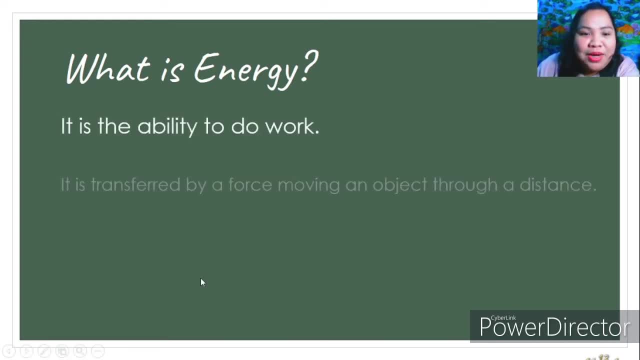 can't do work. that's the simplest thing, okay? so if we say that energy is the ability to do work, um, that means we transfer. we transfer energy by using a force while we move an object through a distance, right, so we transfer energy by using a force, by moving an. 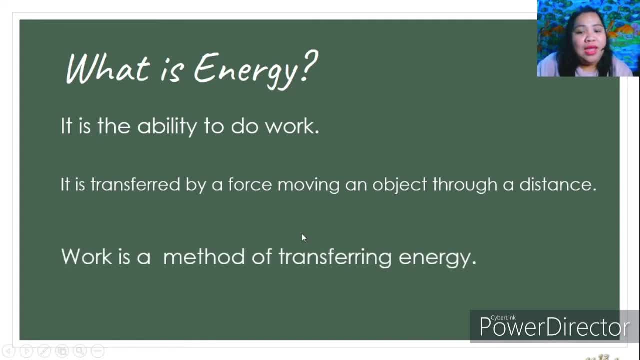 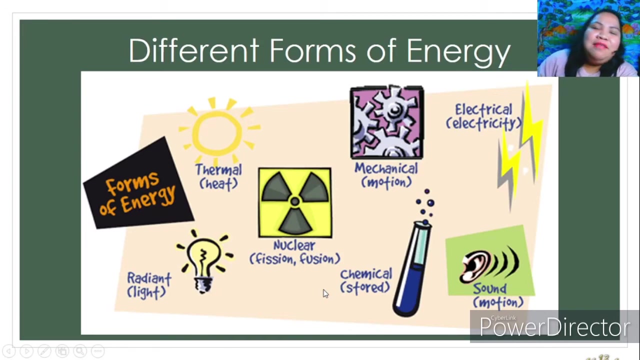 object through a distance. so we can conclude that work is a method of transferring energy. okay, we transfer that energy by using a force as we move the object through a distance. okay, so work, therefore, is a method of transferring energy and energy. speaking of energy, we have different forms of. 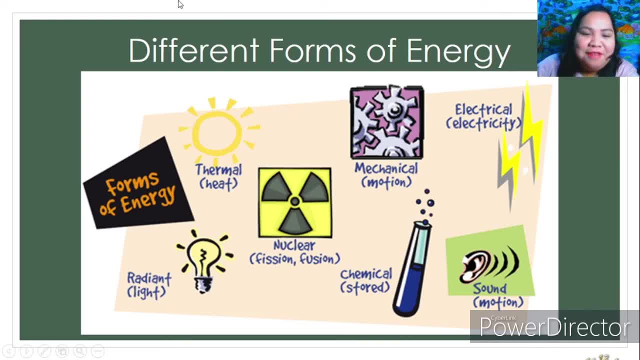 energy. we have thermal energy, we have radiant energy or light energy, we have nuclear energy. we have chemical energy. when we eat something that's chemical energy and our body converts that energy. okay, another sample, another example of energy. we have sound energy, electrical energy and the last one is mechanical energy. okay, so those are the different forms of 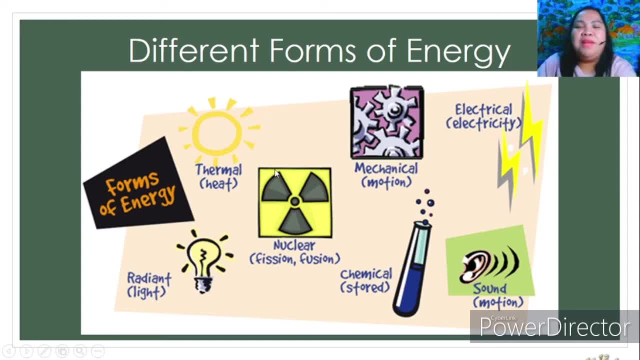 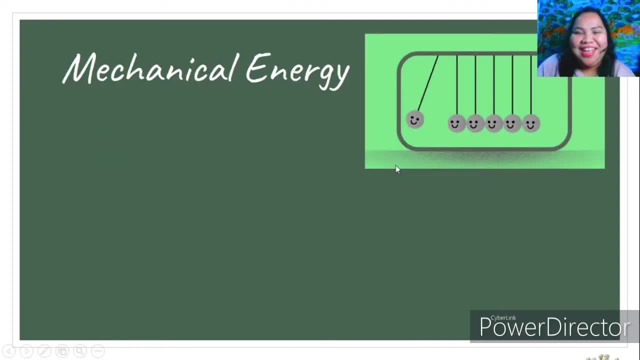 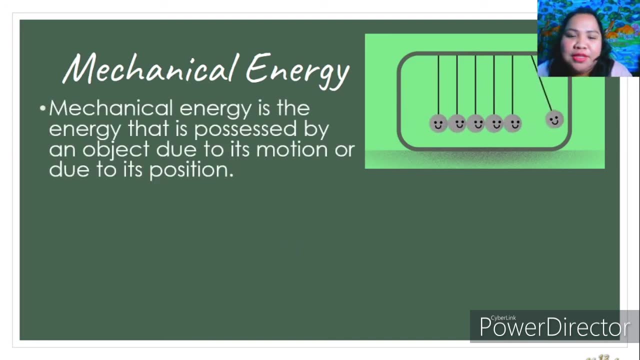 energy. so many of them, but for our discussion we will only talk about mechanical energy. okay, mechanical energy is that energy possessed by an object due to its motion or due to its position, to its position. in physics, this is this, defined as the sum of the potential and the kinetic energy. 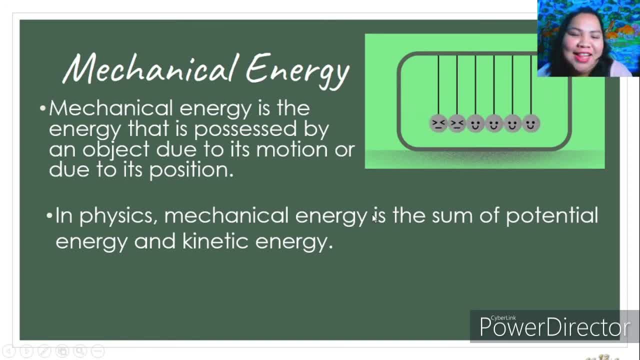 when we say some, we add them up, right. okay. so therefore, the formula for mechanical energy is kinetic energy plus the potential energy. okay, so that is the mechanical energy. it is the energy possessed by an object due to its motion or position, and we have the following formula: kinetic energy plus potential energy. so what is kinetic energy and potential? 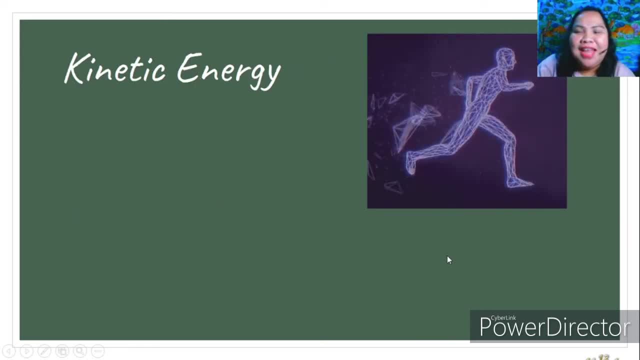 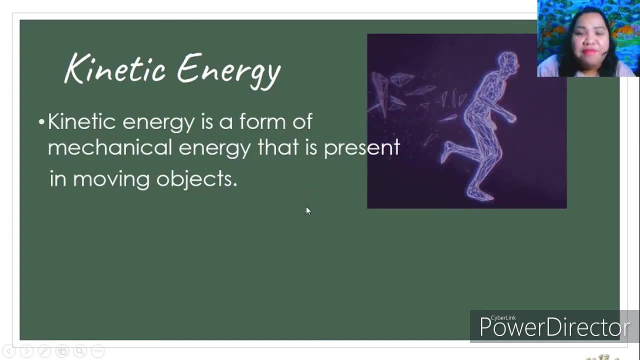 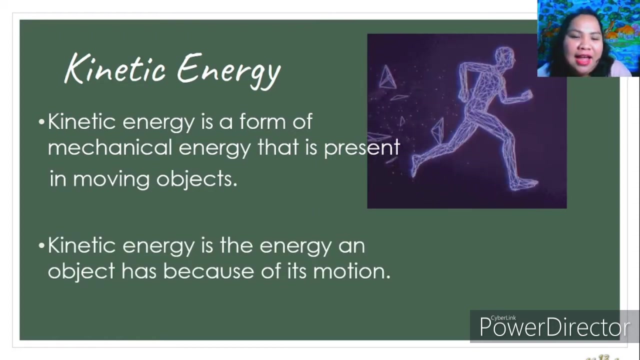 energy. okay, so kinetic energy is- we have an example here- a running man that has so much kinetic energy- kinetic energy is a form of mechanical energy that is present in moving objects. okay, so we can also define kinetic energy as an object. is the energy of an object because of its motion, because it is moving? 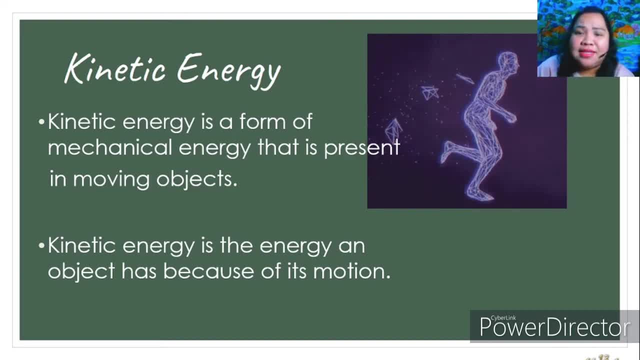 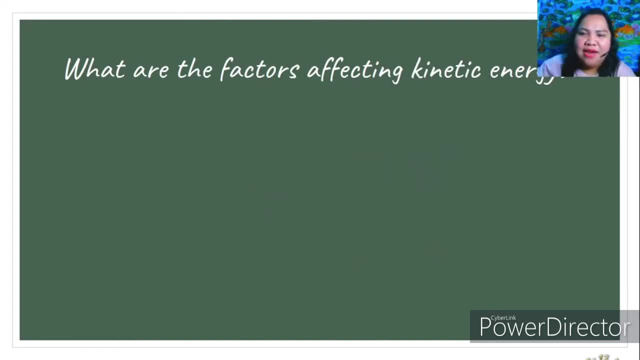 so when an object is moving, it has kinetic energy. okay, so what are the factors affecting kinetic energy? okay, so i have a kinetic energy. okay, so i have a kinetic energy. okay, so i have a kinetic energy. okay, so i have here the following factors: the mass of an object and the speed of an object. 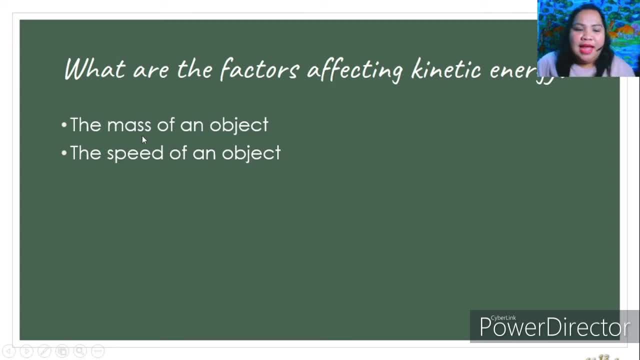 okay. so when an object has a bigger mass, it would really affect the kinetic energy of an object. for example, when we look at a car and a bicycle- okay, so different objects with different mass, okay, we can say that a car would have a greater kinetic energy compared to the bicycle, especially when 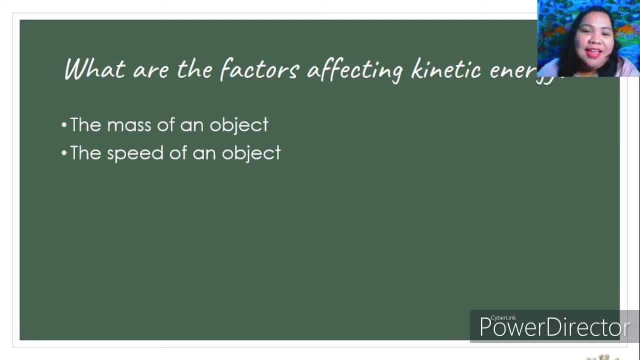 both objects are moving right, okay. at the same time, when the car is moving fast, okay, we have speed here and running faster than the bicycle. therefore the car has more kinetic energy than the bicycle. so two factors that would affect kinetic energy, okay. so if these following factors affect kinetic 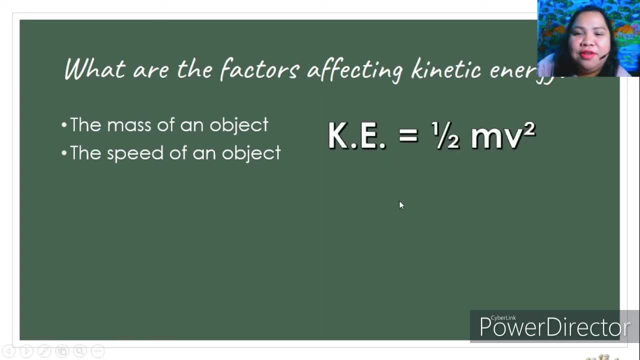 energy. we have the following formula in order to solve kinetic energy. so we have one half multiplied to m and v squared. m stands for mass and v is the speed of an object squared. okay, so also you can use the following formula here, if you are unable to use that one. how to use a? 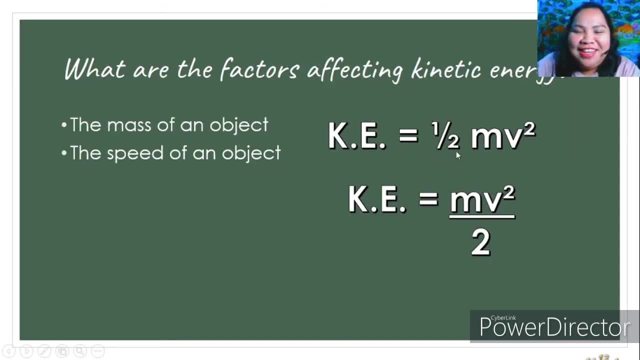 fraction. how to use a fraction in solving that one. okay, so no need to worry, no need to panic. you only have to get the mass of that object and then multiply to its speed, squared, and when you have that product, you divide it by two and there you go. you now have the value for kinetic energy. okay, so so much for kinetic energy. 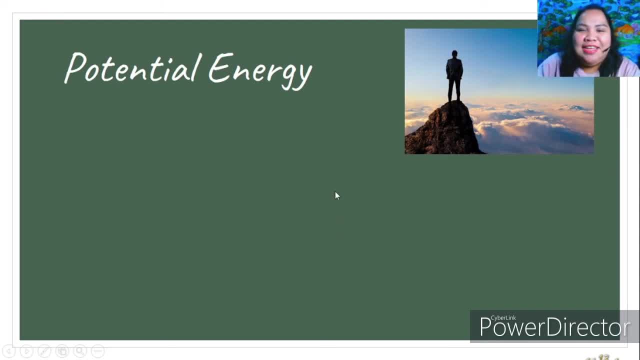 we proceed to potential energy. so now the man who was running earlier is on a top of a mountain. okay, potential energy is a form of mechanical energy that is possessed by an object at rest. okay, when the object is not moving. okay, when the object is not moving. 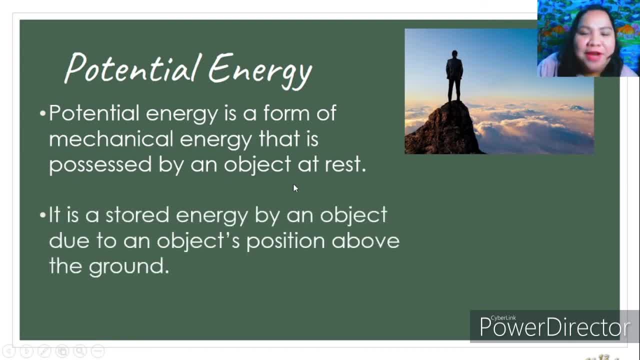 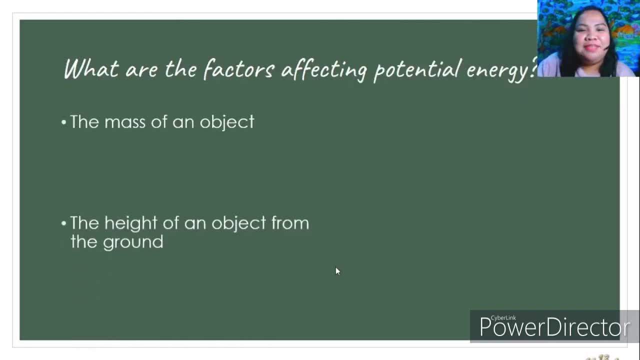 okay. when the object is not moving, it has potential energy. it is a stored energy by an object due to an object's position above the ground. okay, so that is potential energy. okay, so what are the factors affecting potential energy? as you can see, we have also the mass of an object and the height of an object from the ground. so we 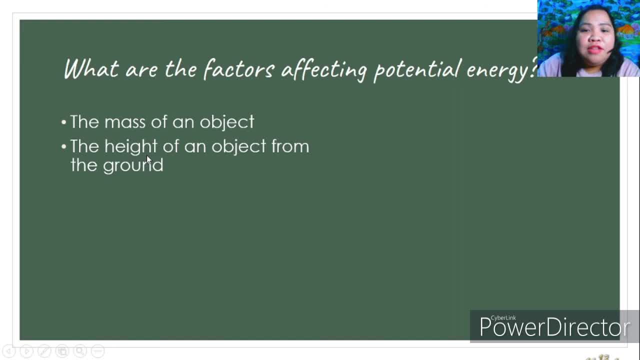 have mass and height and the formula to solve potential energy. okay, so we have mass and height and the formula to solve potential energy. okay, so we have mass and height and the formula to solve potential energy is the following: mgh. where m is the mass of an object, g is a constant value. this is the acceleration due to earth's gravity. 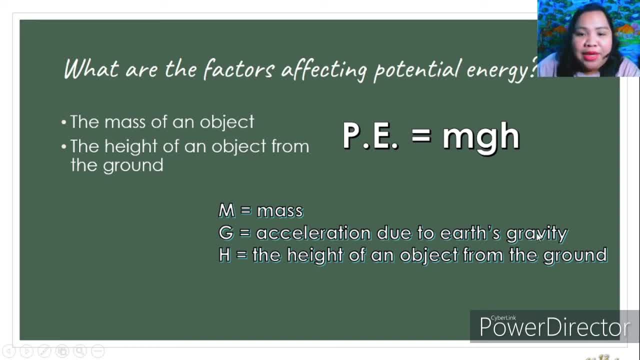 we all know that this is equivalent to 9.8 meters per second squared and the h. the h stands for the height of an object from the ground. okay, so that is the formula for solving potential energy, and the factors affecting potential energy are the mass of an object and the height of an object from the 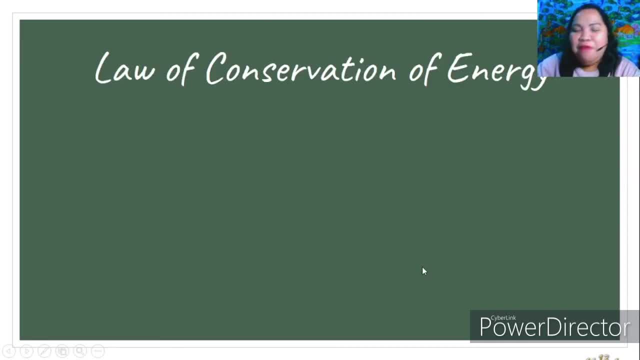 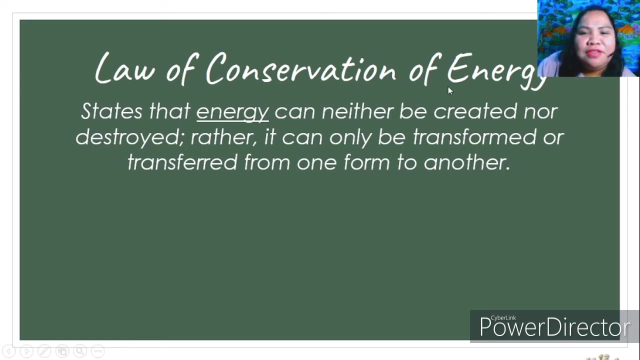 ground. okay, so now we proceed to law of conservation of energy, so that when we say law, it's based on facts. facts, okay, we have evidence, we have evidence of facts. okay, we have evidence to prove that one. so law of conservation of energy states that energy can neither be created nor 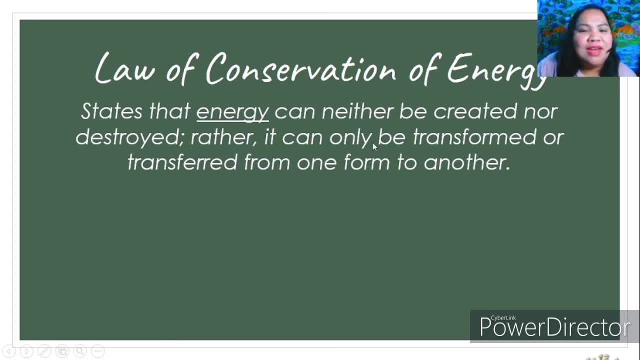 destroyed, rather, it can only be transformed or transferred from one form to another. so it's safe to say that we cannot create energy. energy is stored on different objects, okay, but it can only transfer or transform into another form. so we can also say that a system always has the same. 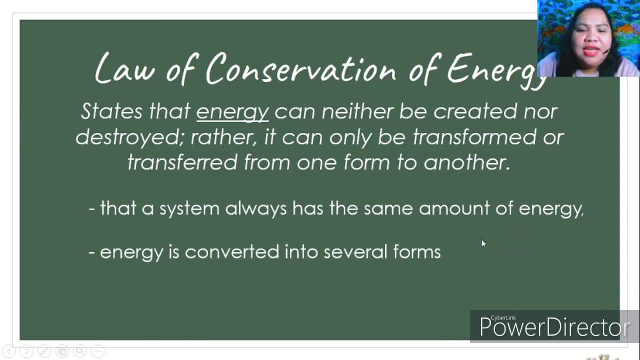 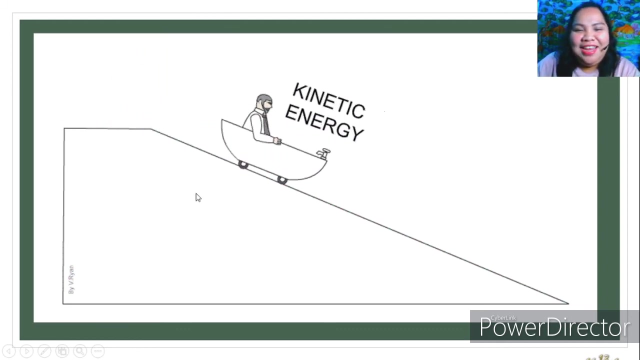 amount of energy and that energy is converted into several forms, but the overall energy of that system will remain the same. it will remain the same, okay. so what is the connection to mechanical energy? okay, so i have here an example: a, a, a, a man on a bathtub, okay, and he's going down, okay, so again, the man on top of that slope has potential. 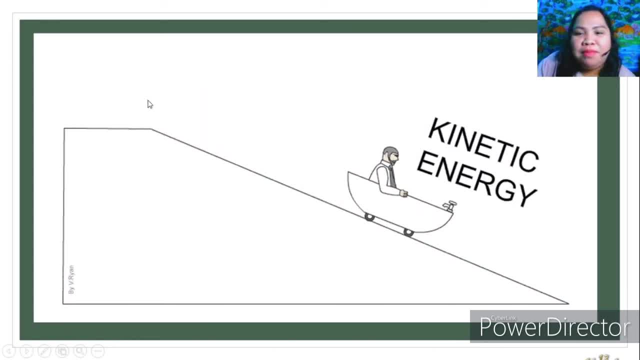 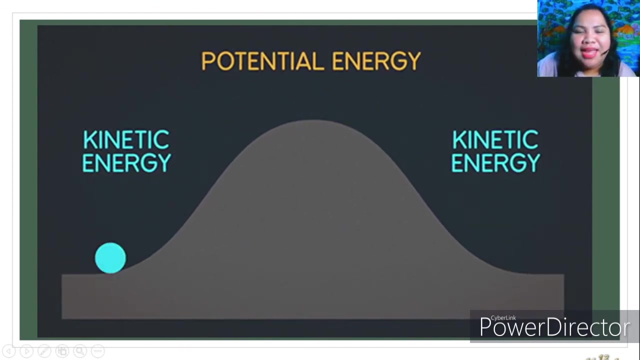 energy because the object is at rest, and when it begins to move downwards, the potential energy is now transformed into kinetic energy. okay, as you can see that. okay, because kinetic energy is the energy of the moving objects. another example here is a ball rolling down a hill. okay, as you can see.